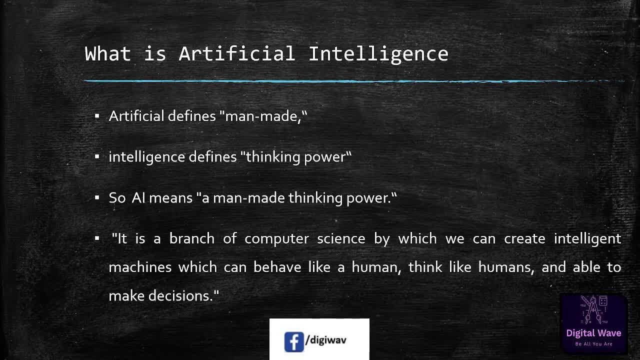 it is a branch of machine by which intelligent machines can behave like humans. this search sign for man-made and intelligent devices has now been established forcibly κ. So think like a human and able to make decisions. AI exists when a machine can have human-based. 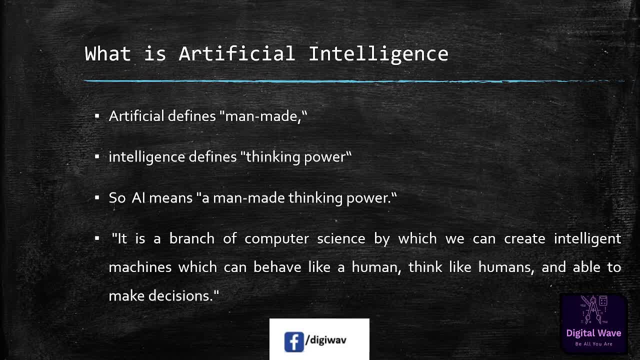 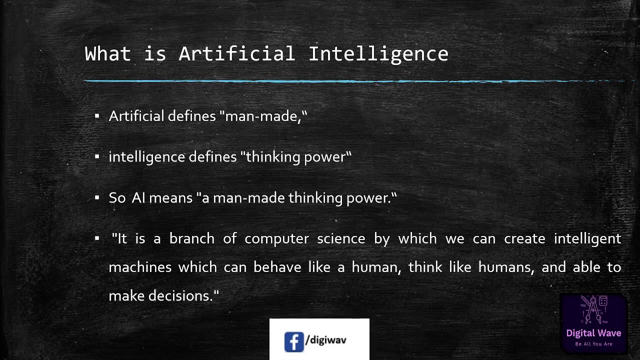 skills such as learning, reasoning and solving problems With AI. we do not need to pre-program a machine to do some work. Despite that, we can create a machine with programmed algorithm which can work with own intelligence, and that is the awesomeness of AI, Or we can say, the science. 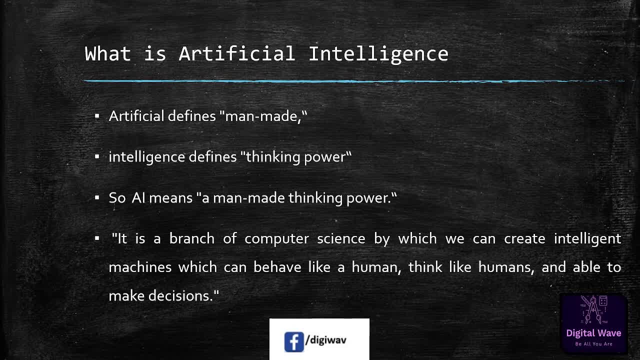 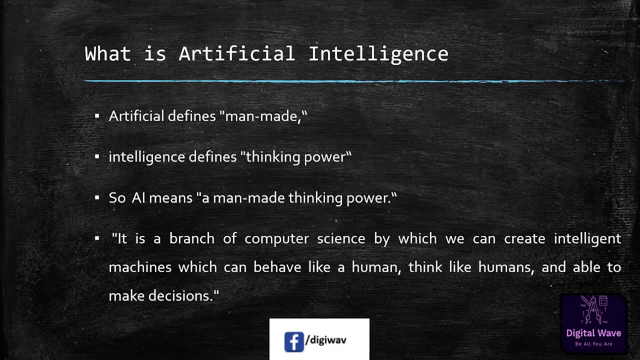 and engineering of making intelligent machines, especially intelligent computer programs. Some of the philosophers also give their philosophy about the artificial intelligence, like while exploiting the power of computer system. the curiosity of human led him to wonder: can a machine think and behave like a machine? 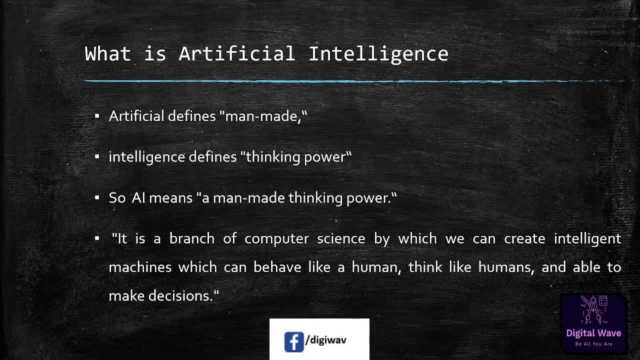 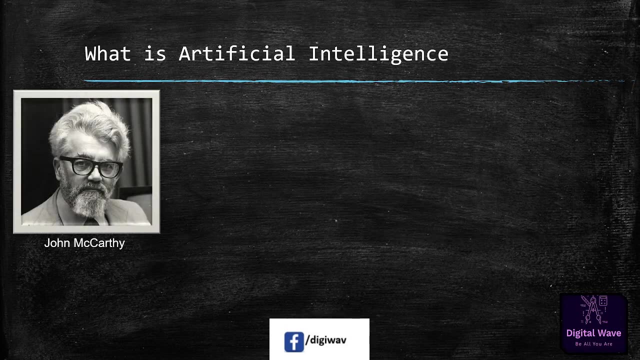 So the development of AI started with the intentions of creating similar intelligence in machine that we find and regard high in the humans, According to the father of artificial intelligence, John McCarty, what is the artificial intelligence? So here the John McCarty said about the artificial intelligence: the science and engineering of making intelligent machines. 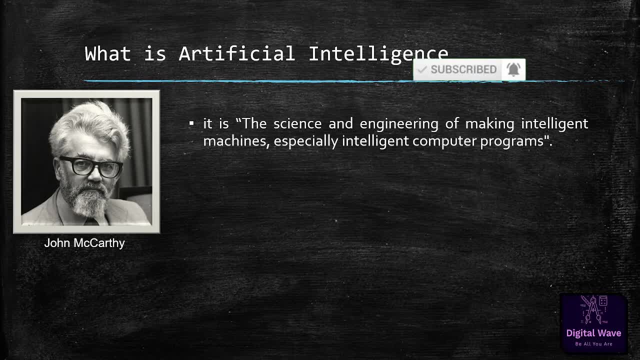 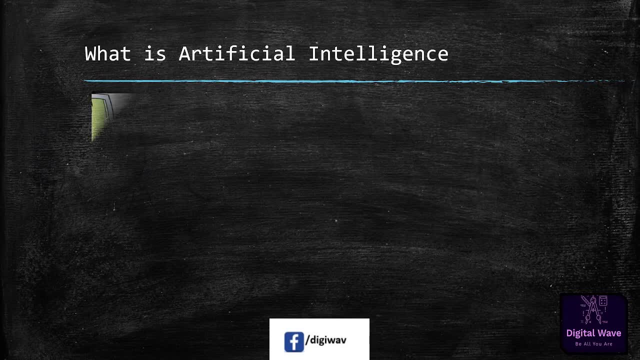 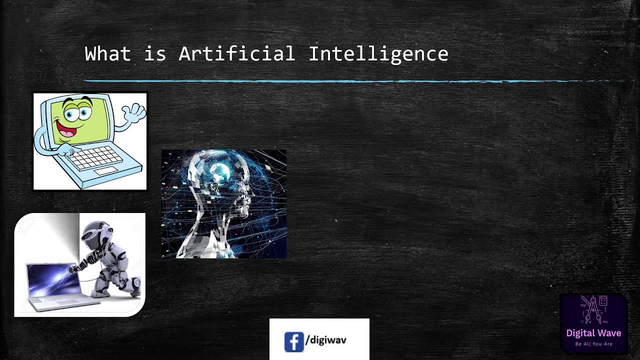 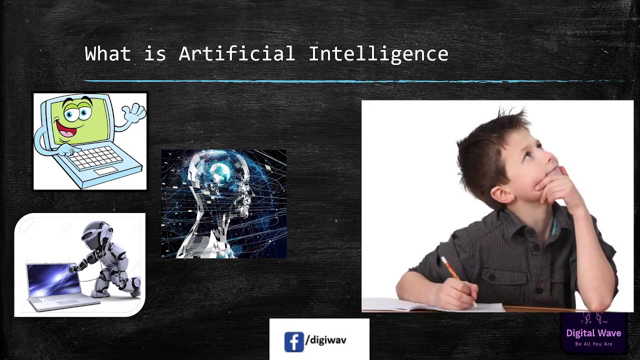 especially intelligent computer systems, are called artificial intelligence. So, as per this statement, we can say that artificial intelligence is a way of making a computer, a computer controlled robot or a software think intelligently in the similar manner the intelligent human think. AI is accomplished by studying how human brain thinks and how 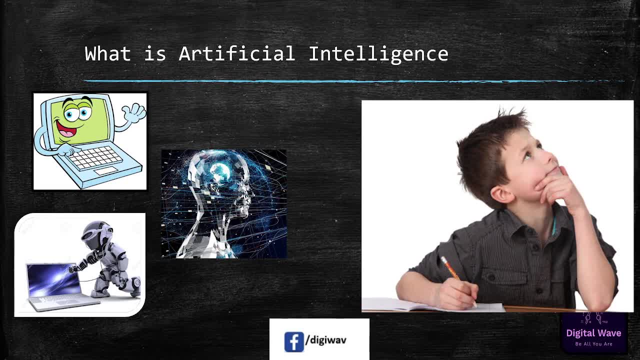 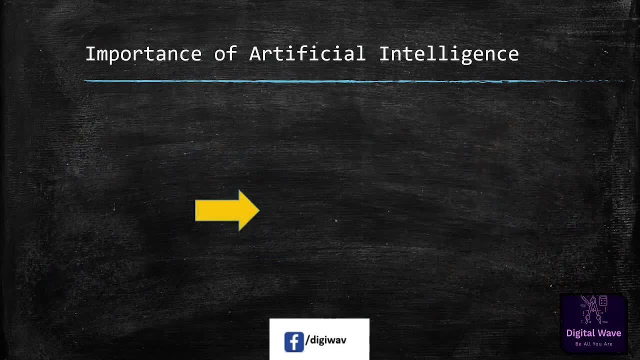 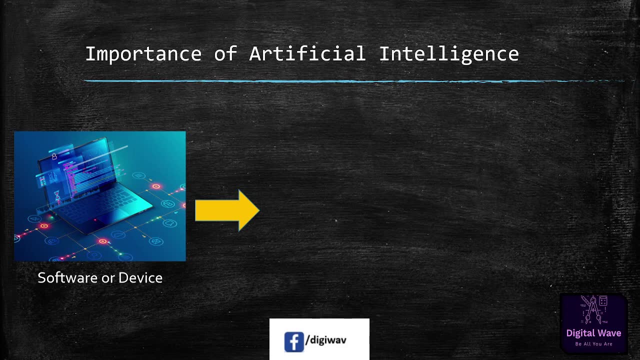 it works while trying to solve a problem and then using the outcomes of this study as a basis of developing intelligent software and systems. So, if you will talk about the importance of the artificial intelligence, so before learning about artificial intelligence, we should know that what is the importance of AI and why should we learn it? So there are 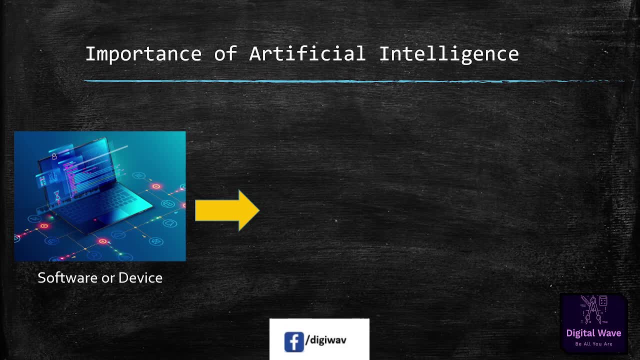 some points we will discuss that will prove that this is the important point. So let us come to the importance of the artificial intelligence in our future. So, with the help of AI, we can create a software or device which can solve real world problem very easily, with accuracy. 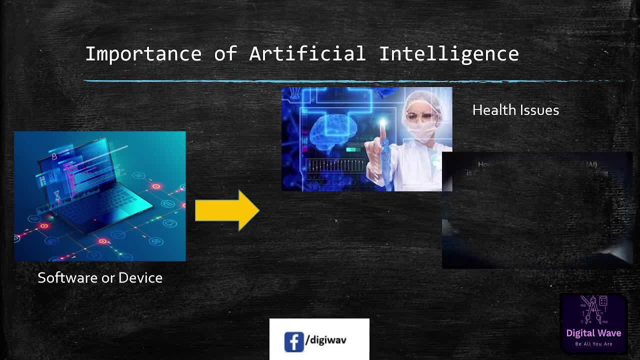 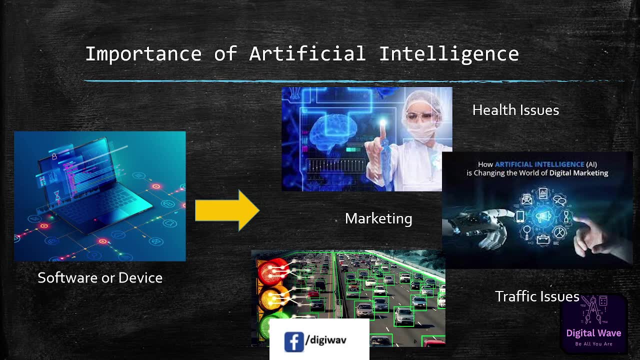 such as health issues, marketing, traffic issues. So these are the some points by which we can provide the solution in this particular sector with the help of artificial intelligence. With the help of AI, we can take solutions out of the felt taken in difficult part. So 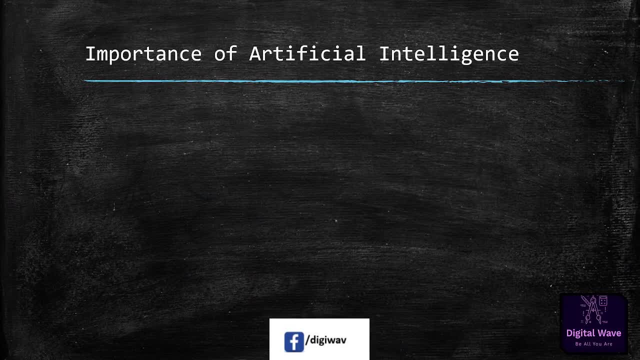 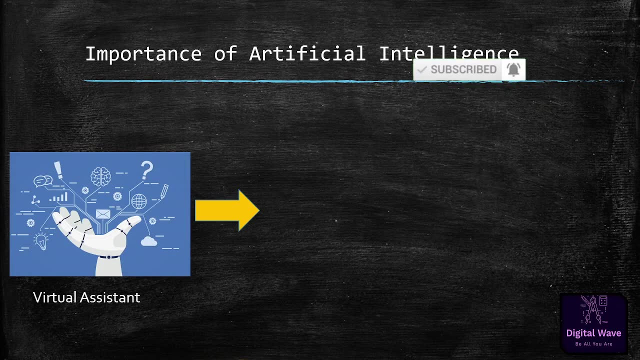 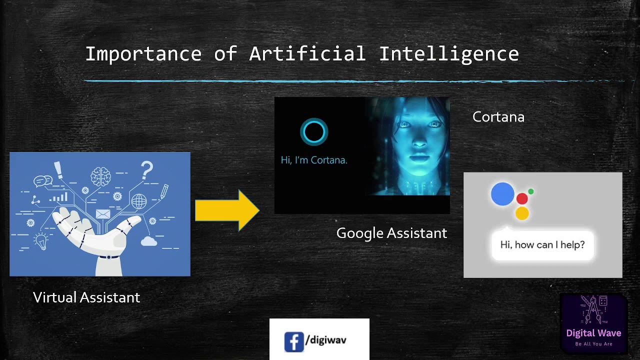 now we will see that what is the real object of AI and what actually it is. after creating of AI, we can create our personal virtual assistant. okay, so what are these personal virtual assistant we can use in our life? so these are cortana, google assistant, siri. these all are personal. 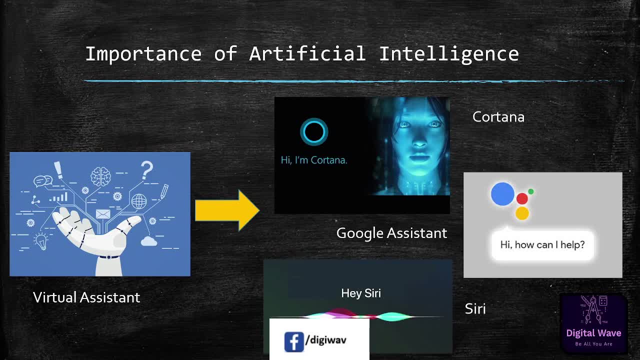 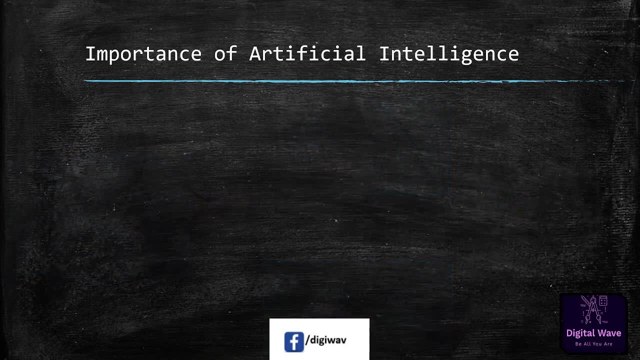 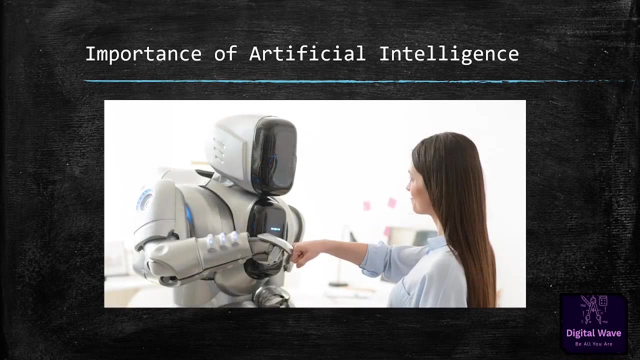 productivity assistant that help us to save time and focus attention on what matters most. with the help of AI, we can build such robots, which can work in environment where several human can be at risk. AI opens a path for other new technologies, new devices and new opportunities. now we will discuss some points about the goals of artificial intelligence. so 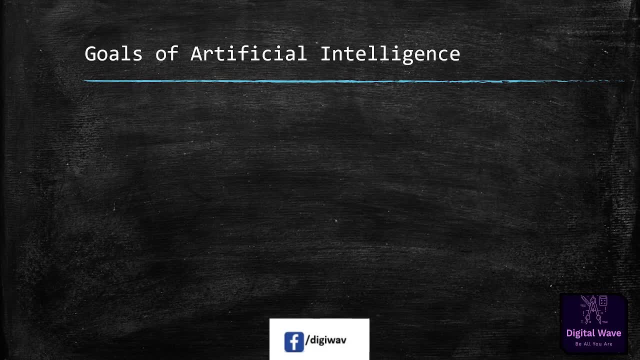 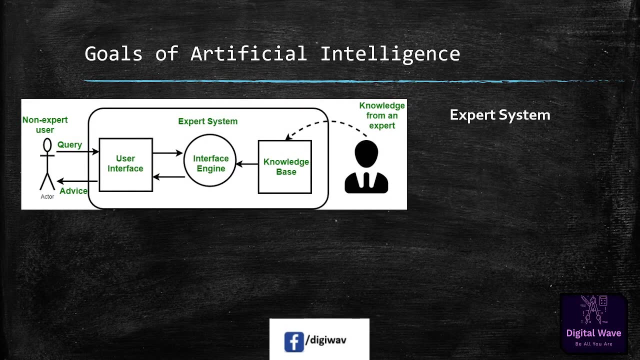 here we will discuss the standard goals of the artificial intelligence. so first is to create an expert system is a goal of the artificial intelligence. so what we can understand by this expert system, the system which exhibit intelligent behavior, learn, demonstrate, explain and advise its user. so this is a very, very important goal of the artificial intelligence. and the second one is: 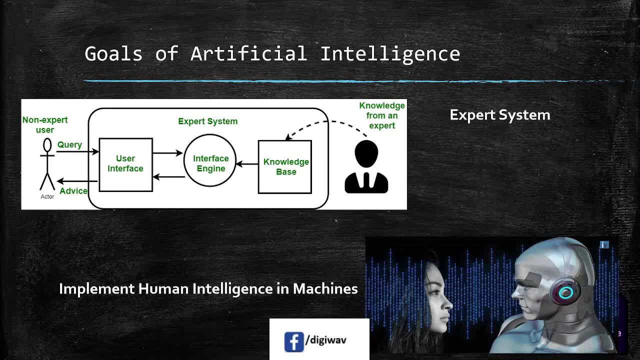 to implement human intelligence in machine, so how we can create human intelligence in machines, so creating systems that understand, think, learn and behave like humans. so this is how we can implement the human intelligence, or we can create human replica in the machines. so there are some points also here to discuss about the goals of artificial intelligence. so we can say that we 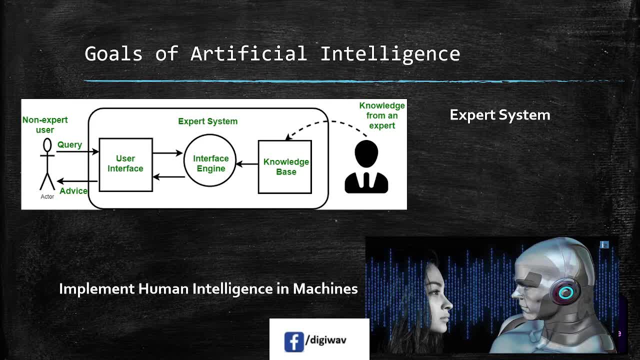 want to create a replica of human intelligence, or we can say we have to solve knowledge intensive tasks with the help of artificial intelligence. an intelligent connection of perception and action is also a goal of the artificial intelligence. and we can say: like building a machine which can, human intelligence, like proving a theorem, playing chess plants some surgical operations. 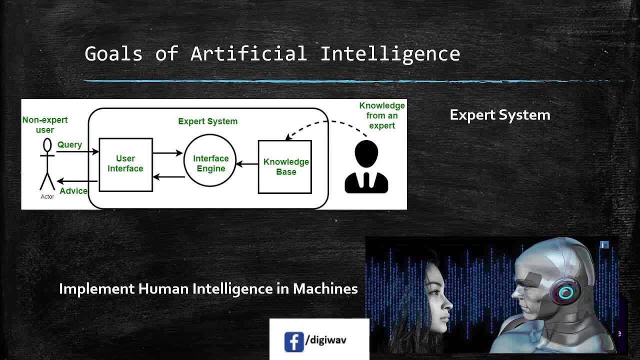 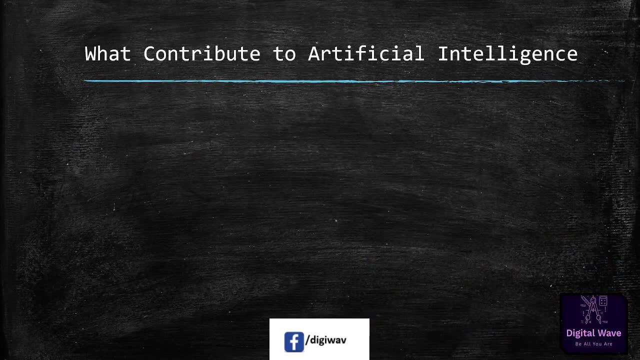 driving a car in traffic. So this is how we can say that we have to create these type of intelligent machines that will be replica of the human brain. Now, in the next slide, we will discuss about the contribution to the artificial intelligence. So here we will see that what? 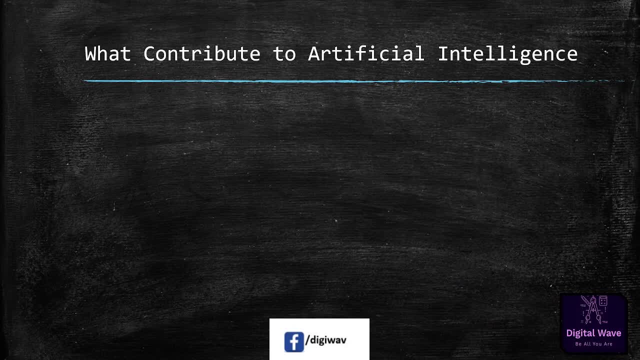 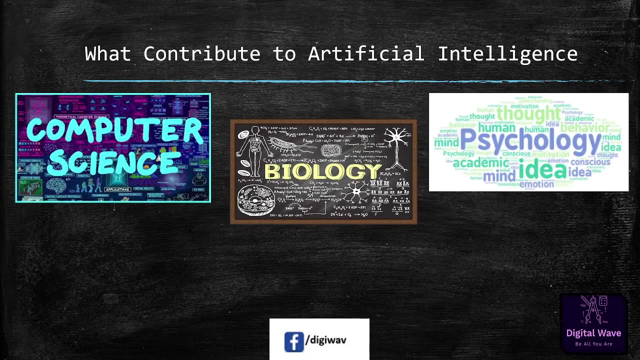 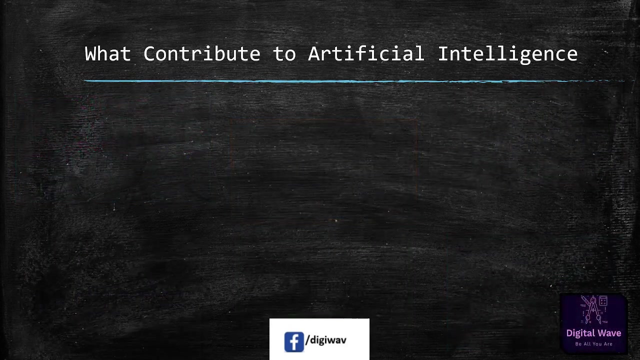 are the branches by which we can contribute something to the artificial intelligence. Artificial intelligence is a science and technology based on some disciplines such as computer science, biology, psychology, linguistics, mathematics and engineering. So we can say: a major thrust of AI is in the development of computer function. 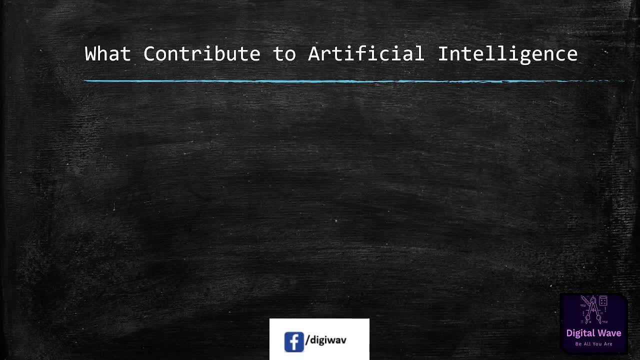 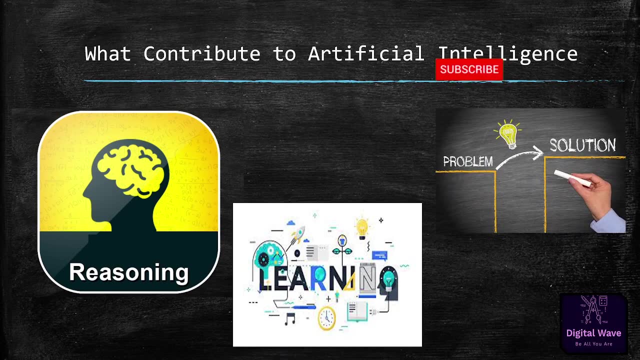 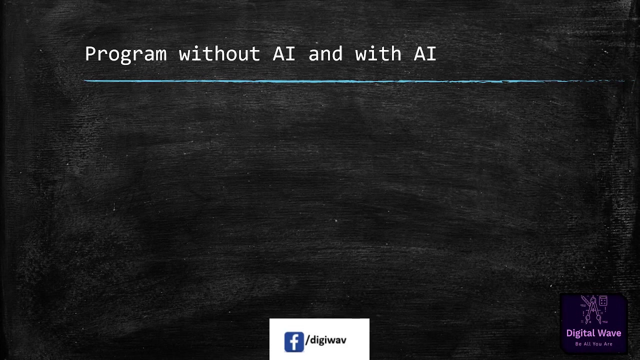 associated with human intelligence, Such as reasoning, learning and problem solving. So out of the following areas, one or multiple areas can contribute to the build and intelligent system. Now, in the next slide, we will discuss that what is the program that is associated with AI and what is not associated with AI? 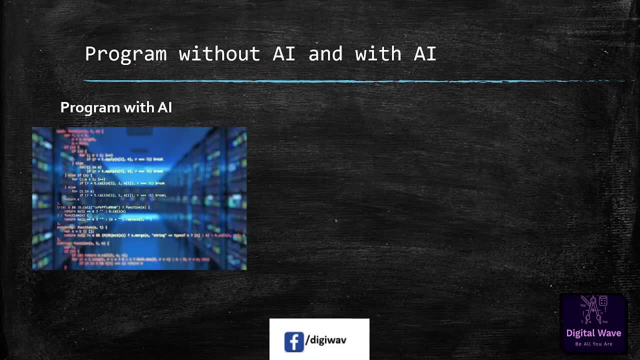 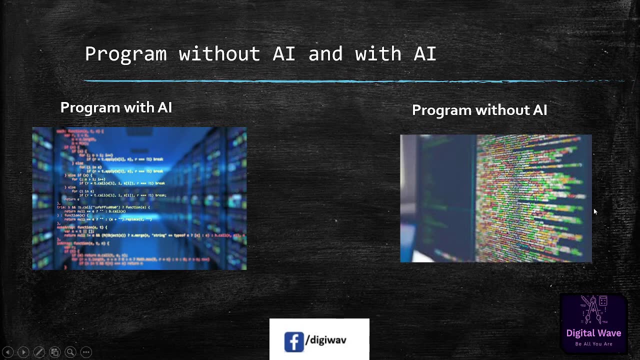 So what are the difference between two types of programs, So with AI and program with without AI? So if we are talking about the program without AI, then a computer program without AI can answer the specific question It means to be solved. Or 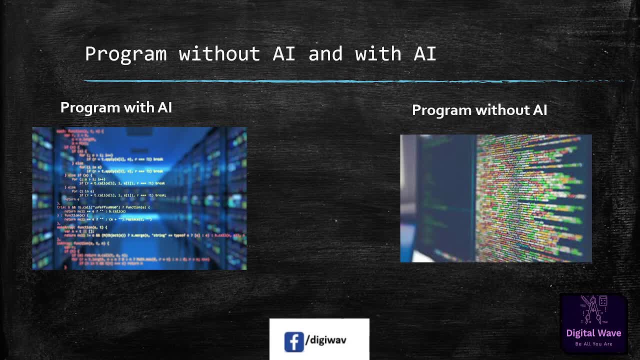 if we want to do some modification in that particular program, then it leads to be changed in its structure. Modification is not quick and easy in the programs without AI, So it may lead to affecting the program adversely Now if we are talking about the programs with AI, so a 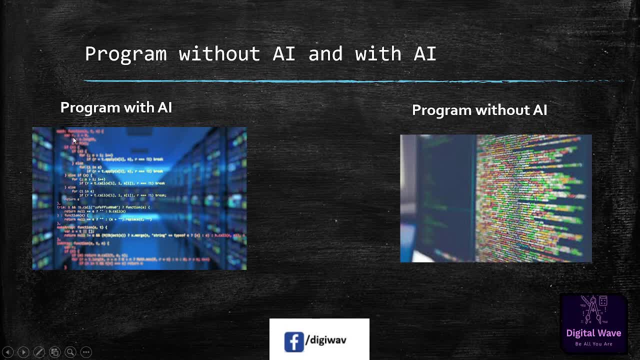 computer program with AI can answer the generic question that means to be solved, And AI program can also observe new modification by putting highly independent piece of information together. Here we can modify even a minute piece of information of programs without affecting its structure. So there is quick and easy modification. 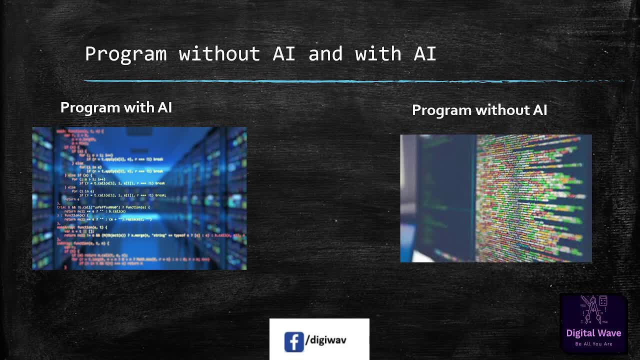 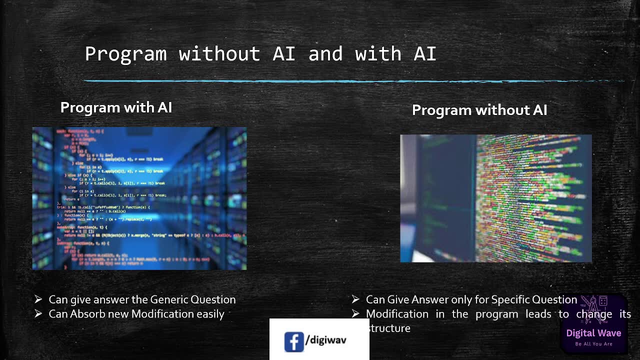 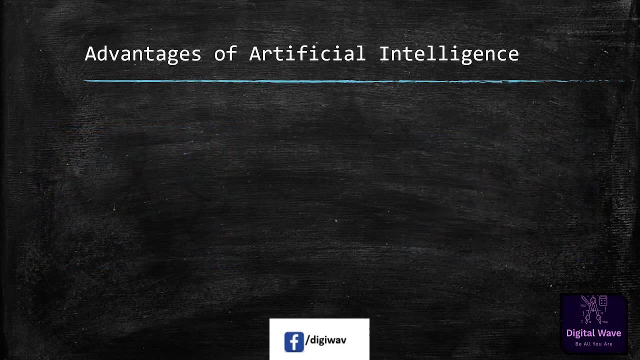 Easy program modification available with program with AI. So this is how we can make difference between program with AI and program without AI. Here we have discussed one or two factors to differentiate both the terms. Now, if we are talking about the advantages of the artificial, 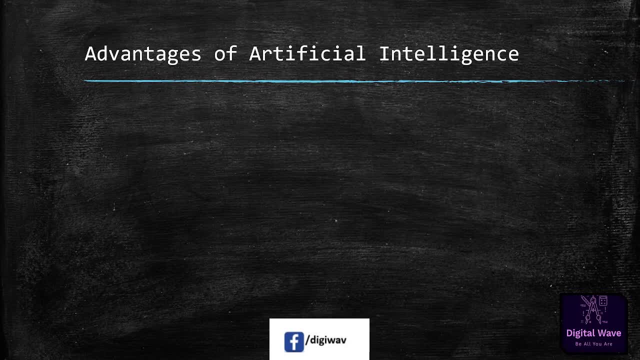 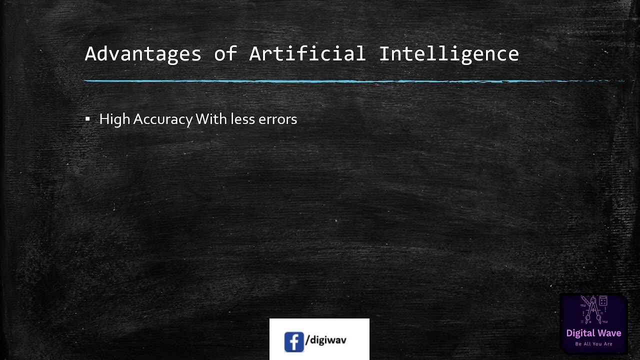 intelligence. so there are many, many advantages of artificial intelligence, But here we will discuss some standard advantages of AI Artificial intelligence. So first advantage of artificial intelligence is high accuracy, with less errors- AI machines or systems are prone to less errors- and high accuracy as it takes decision. 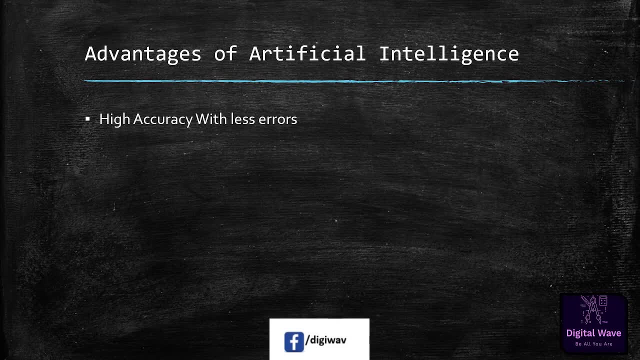 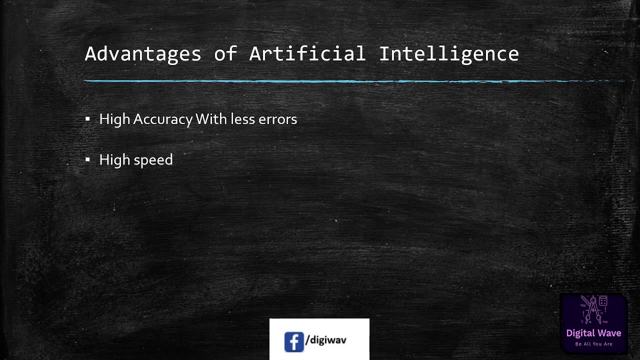 as per pre-experiences or information. Second one is high speed. AI systems can be of very high speed and fast decision-making. because of that, AI system can beat a chess champion in the chess game. Third point is high reliability. AI machines are highly reliable and 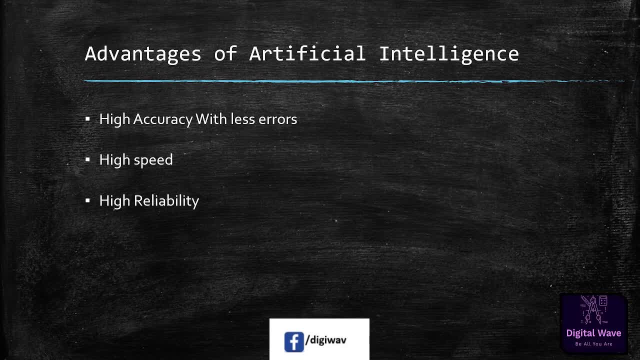 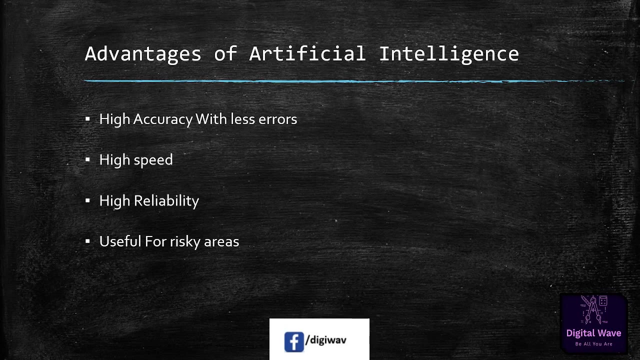 can perform the same action multiple times with high accuracy. Fourth point is useful for risky areas. AI machines can be helpful in situations such as defusing a bomb, exploring the ocean floors, where to employ a human can be very risky. Digital assistant AI can be very helpful when 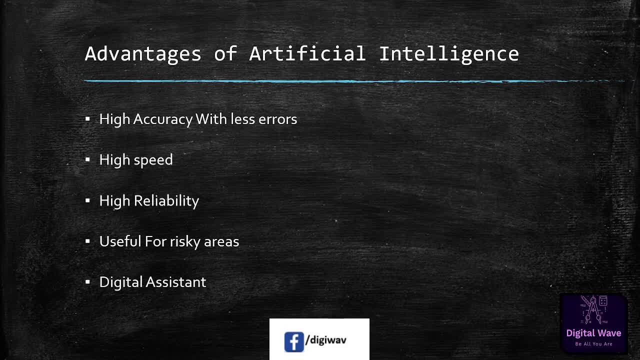 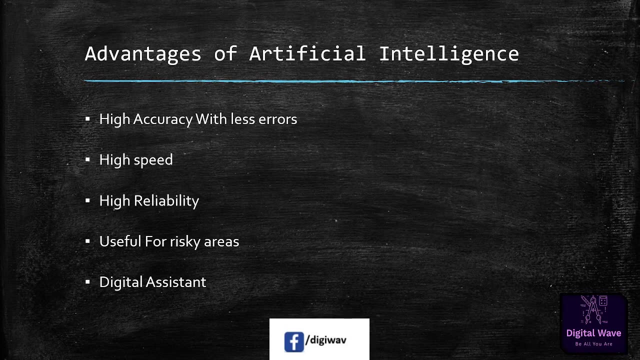 you are in the environment where humans are not easy to get used to, Digital assistant, AI can be very, very useful to provide digital assistance to the users, like as AI technology is currently used by various e-commerce website to show the products as per customer requirements. 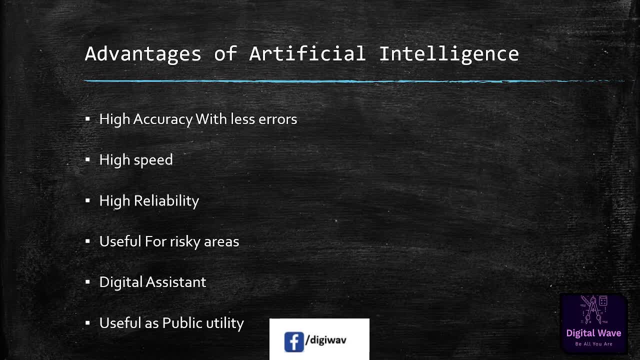 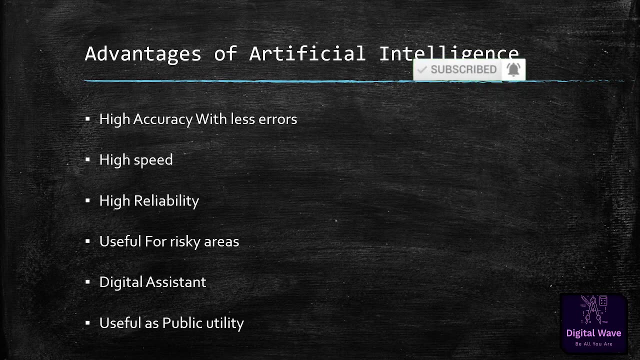 Last point is useful as a public utility. So in this point we can refer like AI can be very useful for public utilities, such as a self-driving car which can make our journey safer and hassle-free. facial recognition for security purpose. natural language processing to communicate with the human in human languages. So there are some advantages we have discussed. 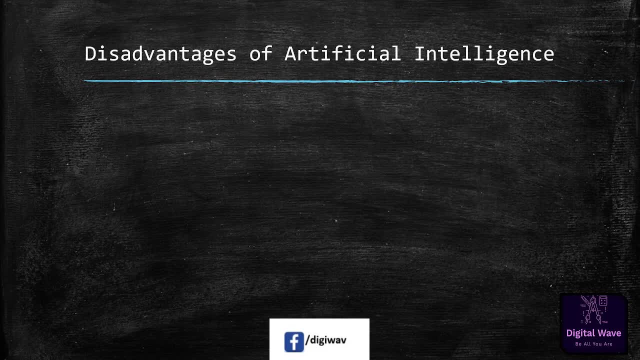 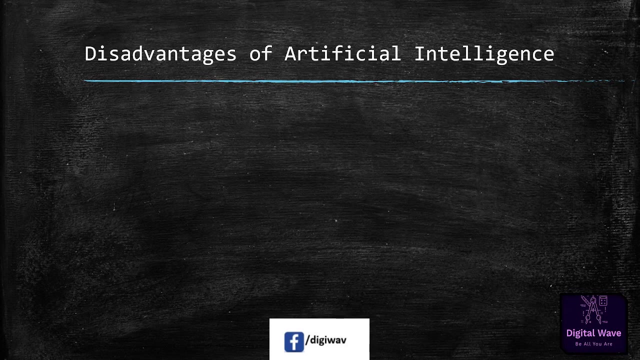 about the artificial intelligence. Now we will discuss some disadvantages of the artificial intelligence. So every technology has some disadvantages, and the same goes for the artificial intelligence Being so advantageous technology, still it has some disadvantages which we need to keep in our mind while creating an AI system. So there are some disadvantages. we are going. 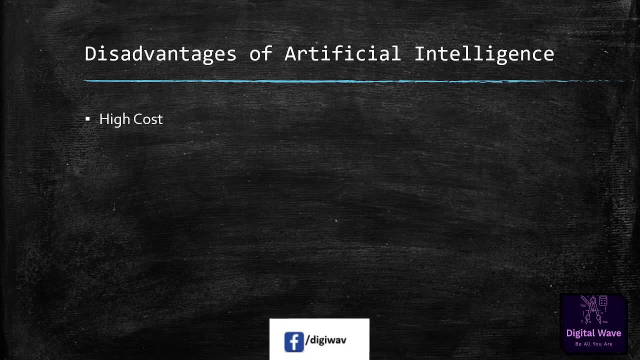 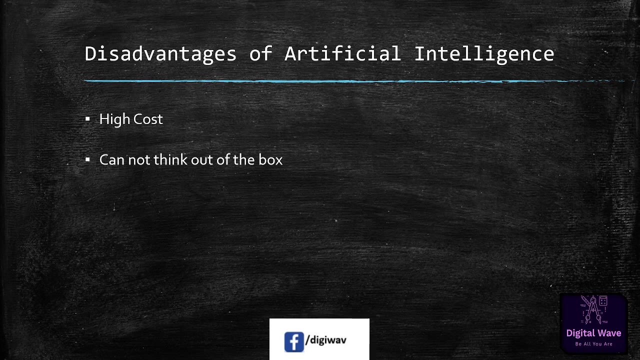 to discuss here. So first one is high cost. So the hardware and software requirements of AI is very costly as it requires lots of maintenance to meet current world requirements. Second point is papaverken AI Network. raw costs means humans cannot think out of the box. Also, we are making smarter machines. 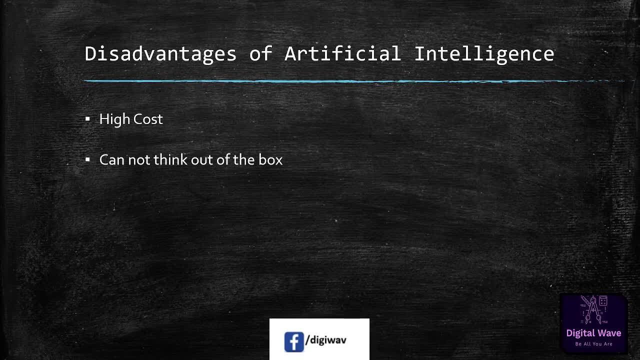 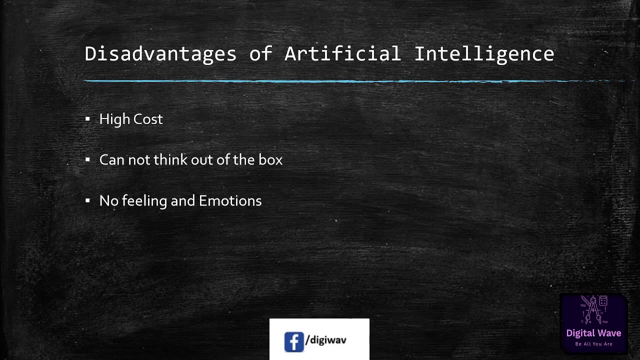 with AI, but still they cannot work out of the box As the robots. only this just does that work for which they are trained or programmed: power processing. Next point is no feelings and emotional AI machine makes everybody happy. They have both raw and balanced emotional connection. AI machines can be outstanding performer, but 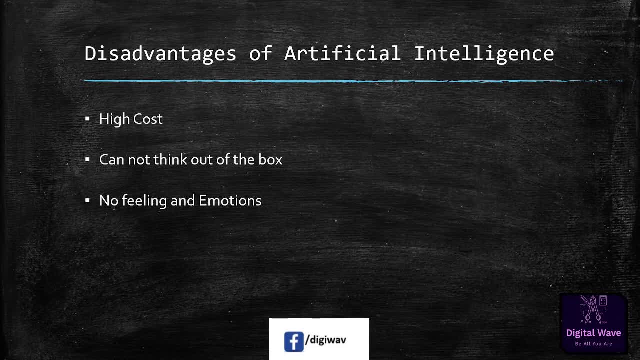 still, it does not have to make emotions in easy mode to crawl, head beta and transform the robot's environment with the world. Baby, baby can not get angry because AI can tonally bounce the hooray human and may sometime be harmful for user if the proper care is not taken. 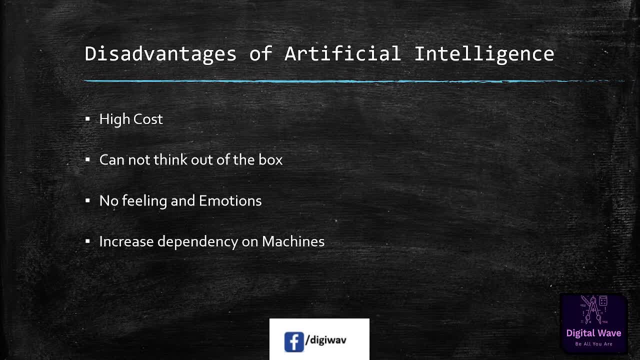 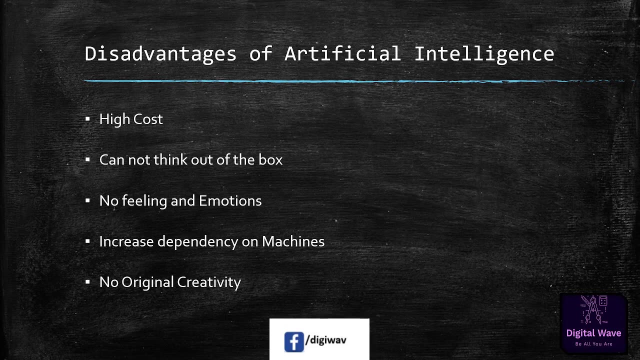 Next point is increase dependency on machines. with the increment of technologies, people are getting more dependent on device and hence they are losing their mental capabilities. Last one is no original creativity. as human are so creative and can imagine some new ideas, but still AI machines cannot beat this power of human intelligence and cannot be creative. 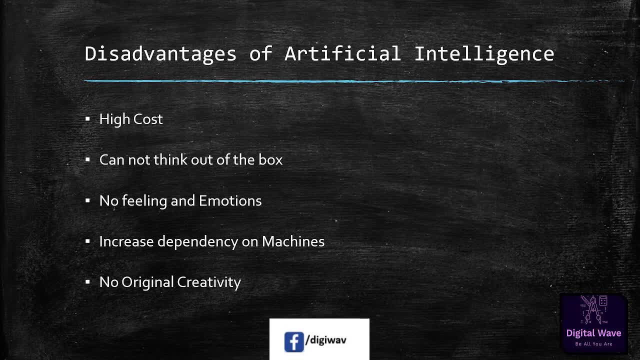 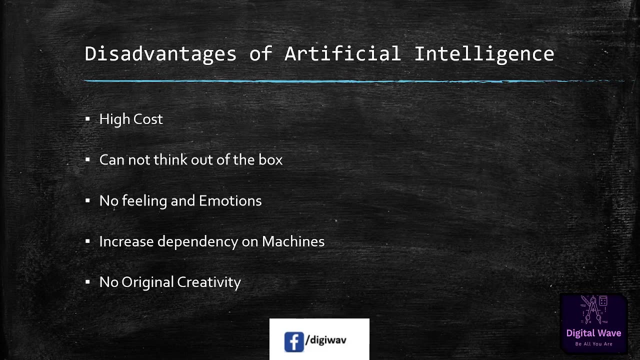 and imaginative. So this is how we have discussed some advantages and disadvantages of the artificial intelligence. So in this tutorial, we have a clear understanding about artificial intelligence. then, what is artificial intelligence and what the future scope or goal, or what are the advantages and disadvantages of the artificial intelligence?